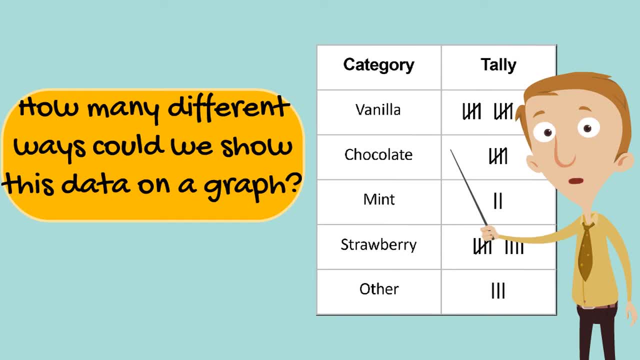 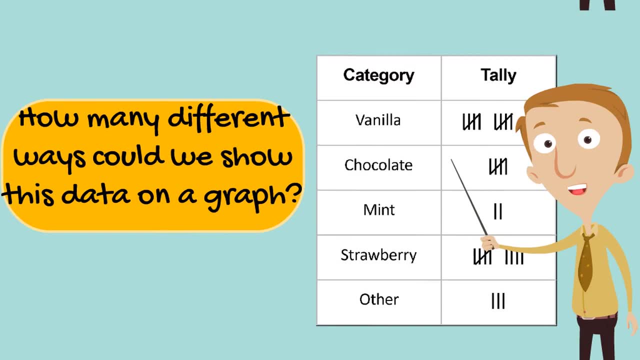 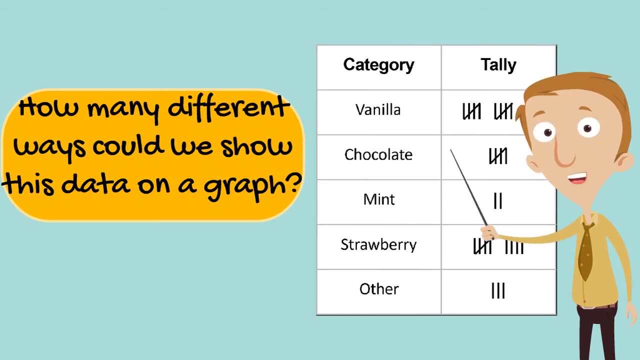 the last week. how many different ways would you be able to show this data on a graph? I can think of at least three different types of graphs you could draw. See if you can think of all three. Pause the video and write down your answers. 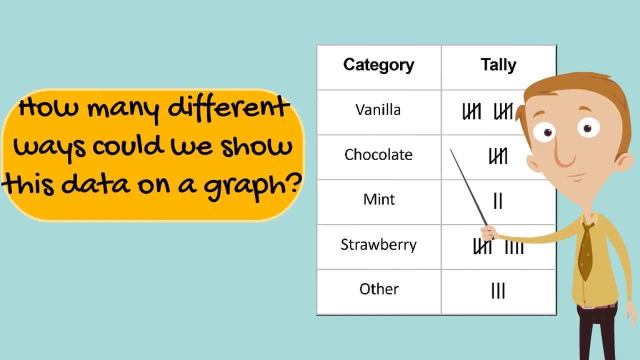 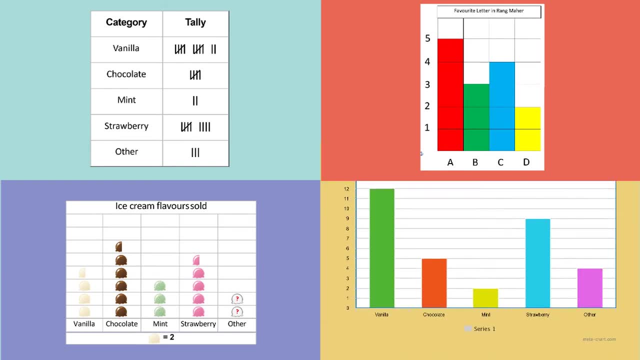 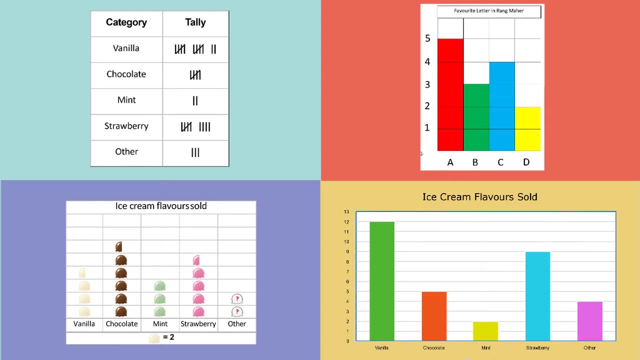 Well, the three different types of graphs we talked about were pictograms, block charts and bar charts. Well done if you remembered all three types of charts. We're going to take a closer look at bar charts today, because they're the most useful type of graph we can learn about. 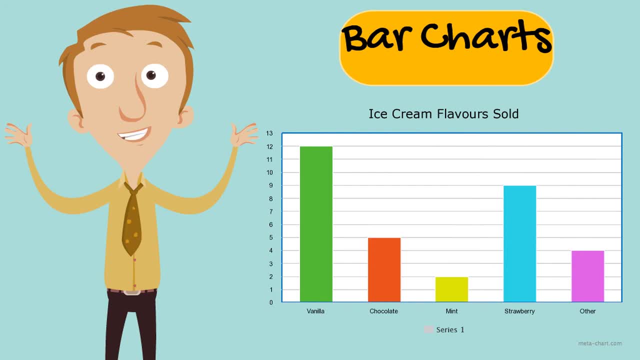 at the moment. So remember from yesterday, bar charts are a little bit different to pictograms and block charts because of the way that we read them. Instead of counting pictures or counting blocks, we read off this numbered scale. Let's take a closer look at our ice cream bar chart. 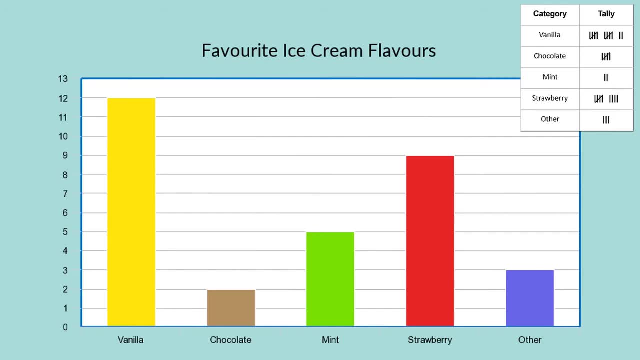 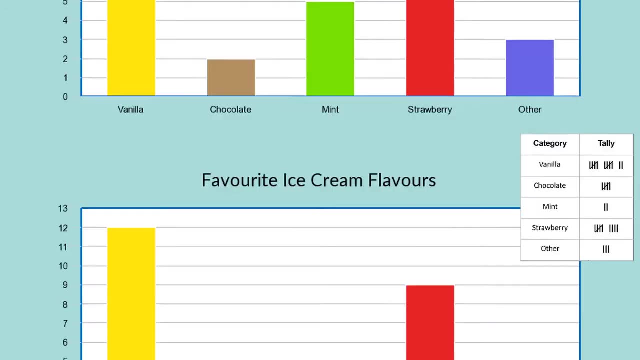 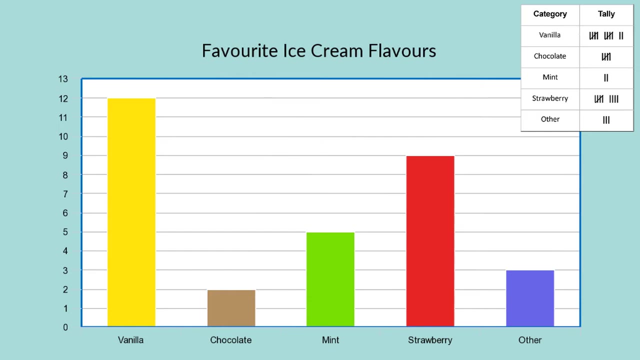 Okay, so here's our tally. That's all correct. Oh, I've made a mistake. There is one One mistake on this bar chart. somewhere I've done something wrong. Can you pause the video and find where I've made my mistake? Use the tally to help you. Pause the video when you're ready. 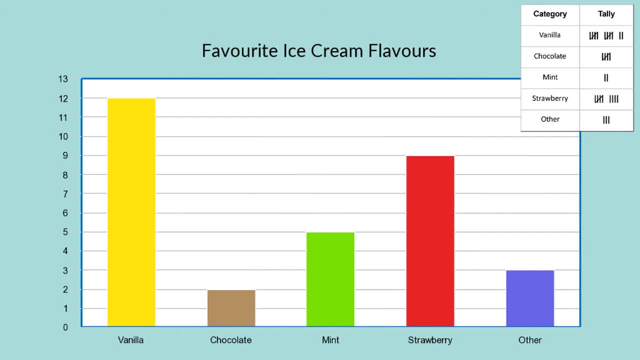 I hope you noticed before I did I mixed up the chocolate and the mint bar. They should look like this instead. That's better Now. now we've got a proper bar chart that's accurate. Remember from yesterday. every bar chart has got a title, it's got a numbered scale, it's got bars and it's got labels. Now here's the. 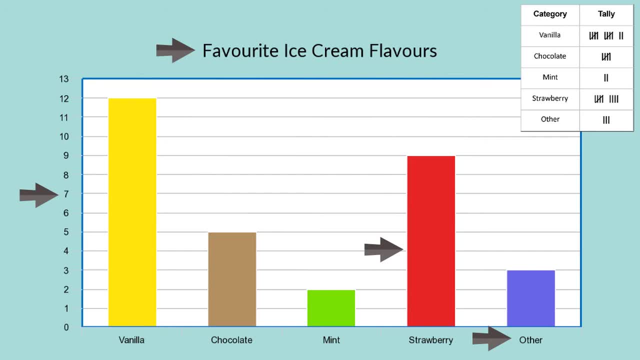 advanced class, the extra piece of information for today's lesson. This is very, very fancy maths language we're learning here. As well as those four important parts, we're going to take a look at the parts, There are two extra ones I want you to remember. Every bar chart has got an x-axis, that is: 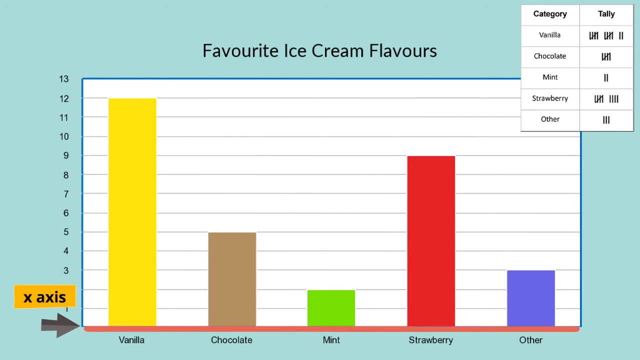 the line that goes along the bottom and a y-axis, That's the line that goes up to the top. The way to remember this is a capital, Y is a tall letter, so it's the tall line, whereas an x is not tall. 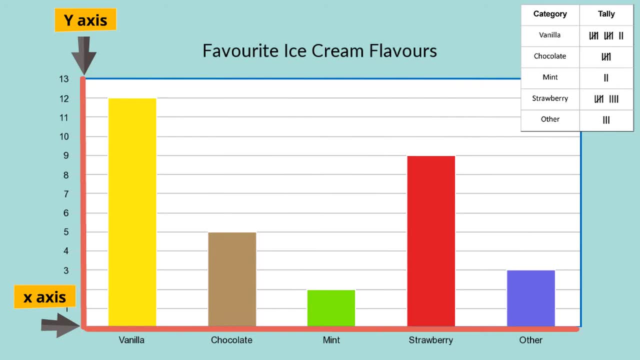 so it's the not tall. When you're drawing your own graphs, you'll have to draw the x and the y-axis yourself. I wonder if you already know how to draw a bar chart properly with all of the parts. Say, an alien popped up and for. 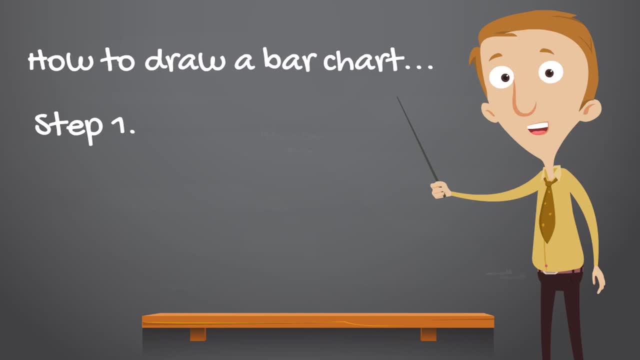 some reason they really wanted to know how to draw a bar chart. I don't know what they want it for, but they really want to know What step Would you give them in the simplest possible instructions? Pause the video and write down. let's say: 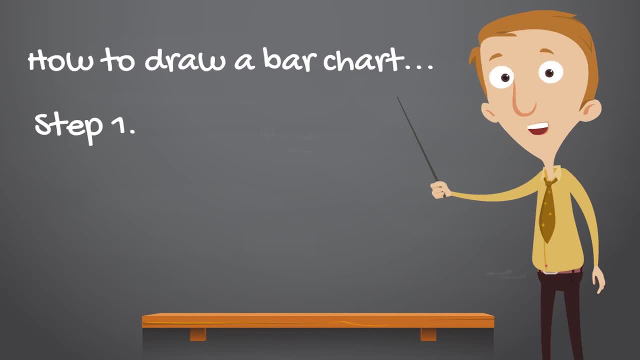 five steps of how to draw a bar chart and try not forget any of the important features. Pause the video and try right down the five steps. Go through the steps and see if you managed to mention all of them. First up, you need some data. Without data, 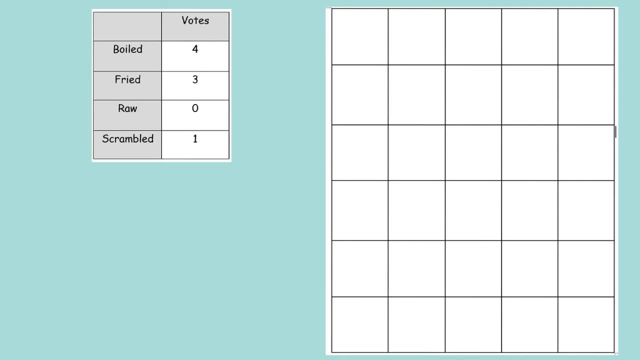 you can't draw anything. When you've got that, the first thing you want to do is draw your x and y axis onto your paper. Make sure your lines are nice and straight. Second step: take a look at your data and write your number. scale up the y axis. Step number three: write your labels under: 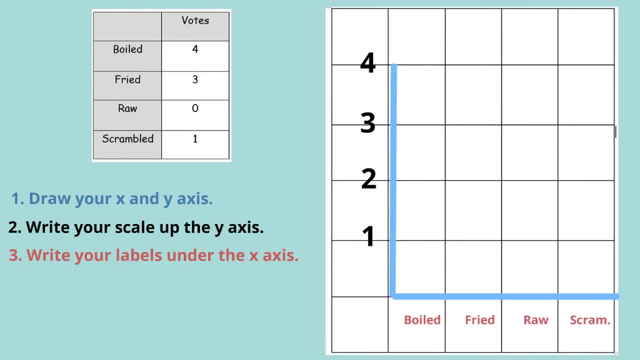 the x axis. Step four: using a ruler, draw your bars using the data on your chart, as neatly as you can Remember. only go up as high as the number on the chart. And number five, write your title up above the bar chart so everybody knows what it's about. And that's how you draw a bar chart Did.